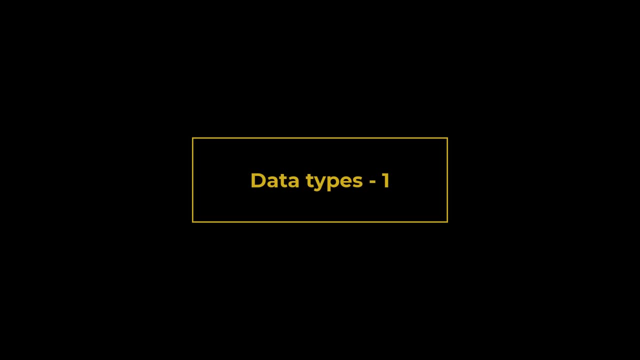 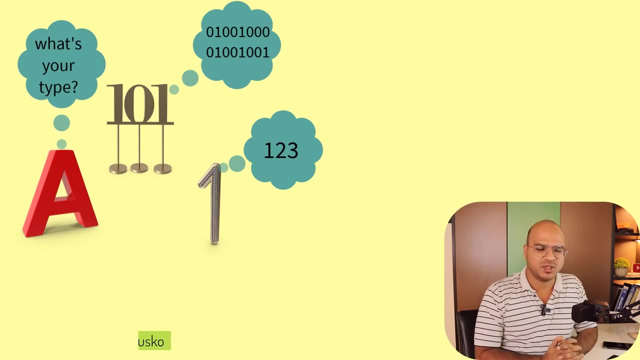 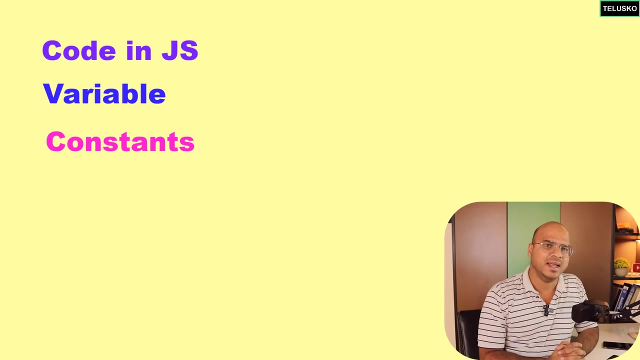 Welcome back aliens. my name is Devin Reddy and let's continue this series on JavaScript. So in the earlier videos we have talked about how to write a JavaScript code, we have seen how to write variables, how to work with constants. It's time to understand one of the most important. 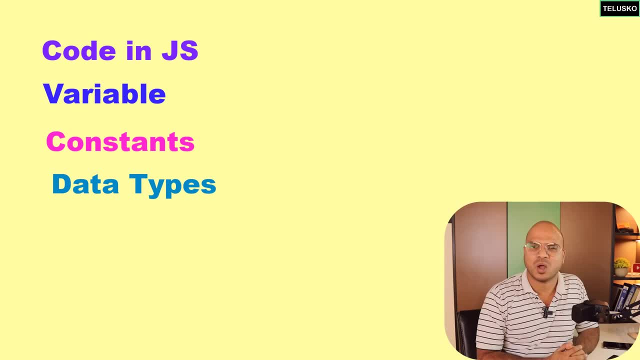 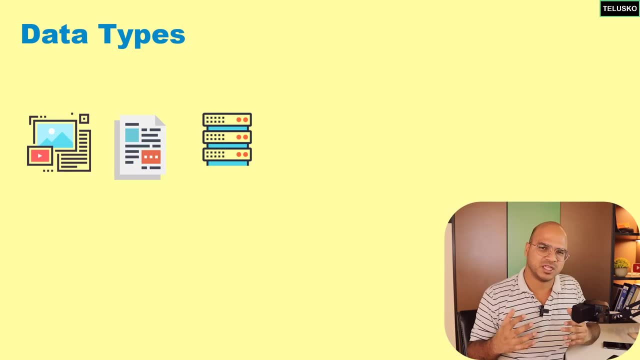 concepts in a language which is data types. Now why it is important. As I mentioned before, the most important thing in any software is data right, Because most of the application we build, we build it for the data, To store it, to process it, to make something meaningful. 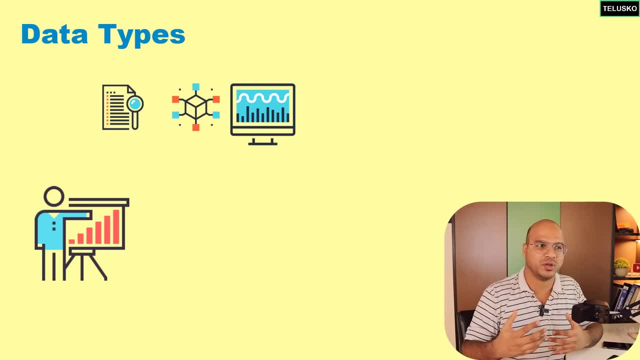 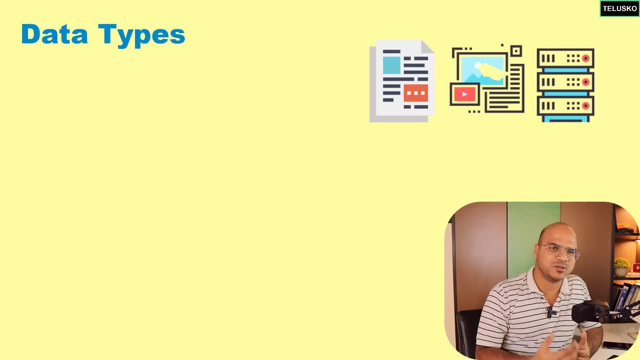 out of it. Maybe if you want to create a graph, if you want to make a game as well. it's all about data right Now. when you are talking about data, it's also important to understand the type of it. Now, what I mean by type. if you remember, in the earlier videos we have, 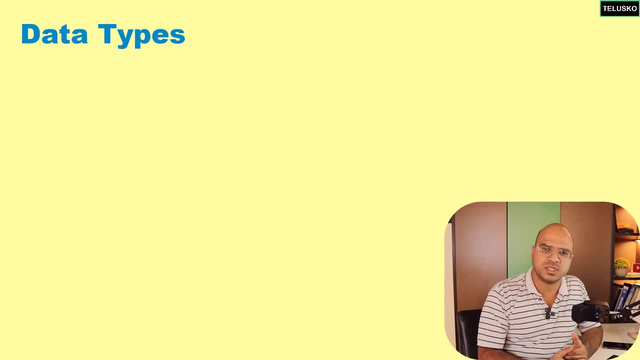 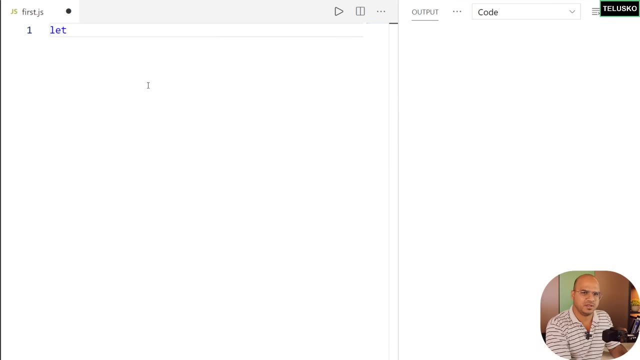 talked about. we can add two numbers, right, And then we can do those things. we can add them. we can find something specific about data based on their type. Example: let me take a variable here and we'll name that variable as data And let's say the value of data is: 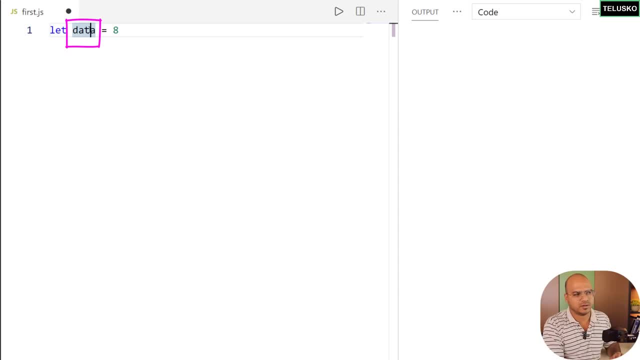 8,. okay, Now, this is a variable. right, We know about it And this is our value. Now, this value will have a type. Now, if you are coming from other language where you define variables and you also mention the type of it, Here, in this case, we assign the type. 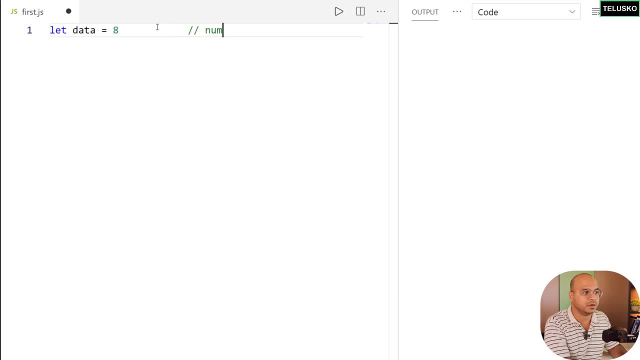 to a value. Now, this value here is of type, number, right? Okay, so that means we can have a number type. What about? let's say, I want to store my name here, So in this case I can select user equal to. I can even have my name here. Now, this thing is a string. So let's say, if we talk, 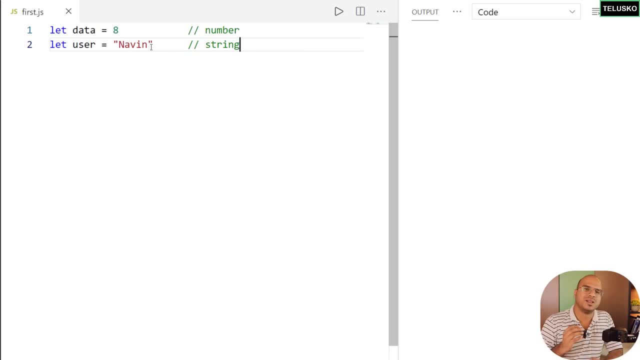 about text. we can call it as string type, So this is what we call as types. So this data here represents a type. Now in JavaScript, basically, you can divide this type into two categories. So you can divide data types into two parts. 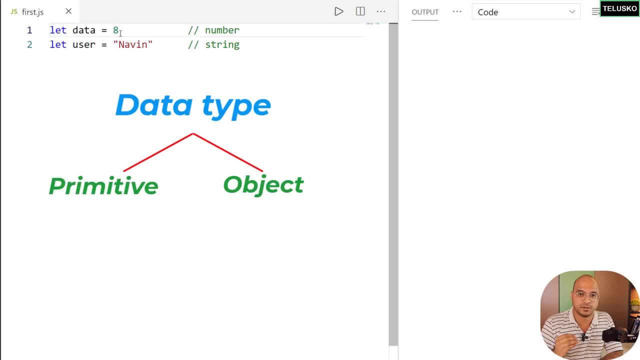 First is primitive and second is object. We will not be talking about everything in this video. There is something which we'll see later, of course, because we have not seen the advanced part yet, And if I talk about those things now you might get confused. 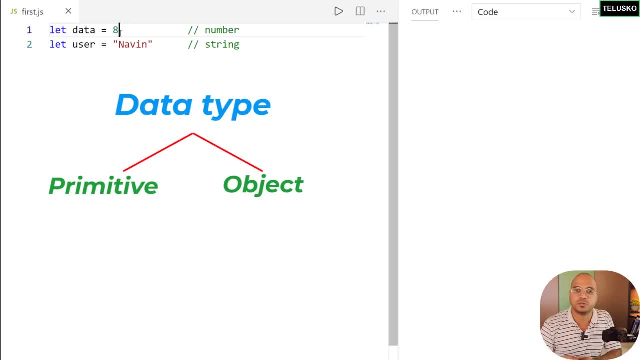 So we'll go step by step. So basically the type is divided into two parts: One is primitive and one is object. So in primitive we have number, string, boolean, null, undefined and symbol. Now, symbol is something which came recently. 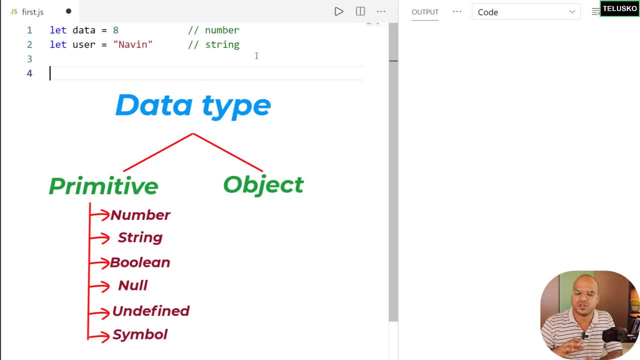 So we'll not be talking about much about that in this video. We'll talk about the numbers. We'll talk about string, boolean, null and undefined, Now whatever is not primitive. So, example: if you have a value which is not a number, which is not a string, which 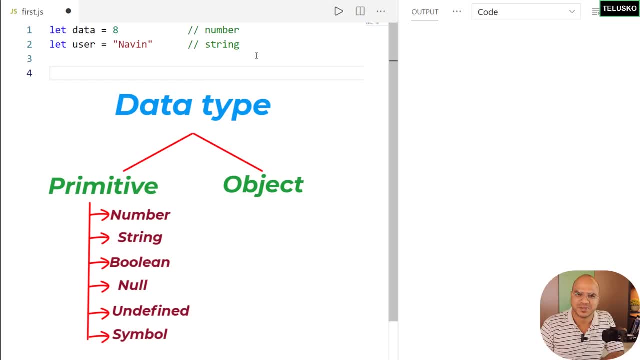 is not a null or undefined, it's an object. Okay, So it's a very complex topic to understand the object part Complex at this point. Once you go ahead, once you understand the basics, it's very easy, Trust me, You know I always follow this line, said by someone very famous. 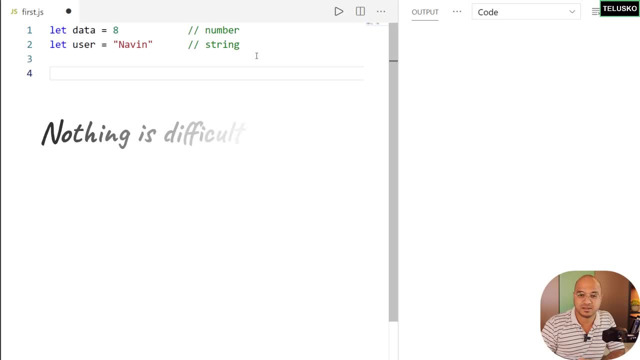 I don't recall. but the statement is: nothing is difficult, It's just unfamiliar. So you just have to get familiar with the language and it's very easy. Okay, so let's start with numbers Now. numbers are numbers, right. So whenever you have a number, let's say 8,, 5,, 15,, any 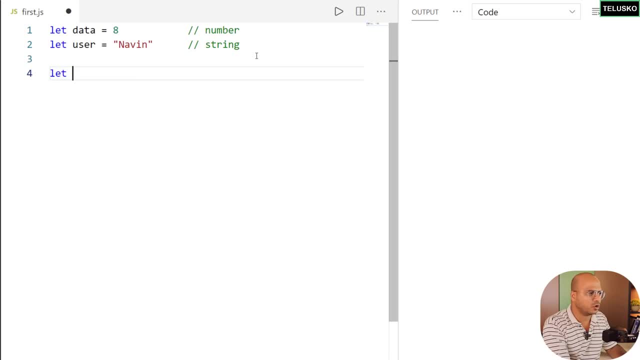 big number doesn't matter, It's a number. So in this case I will go for a bigger number now. So I will say now 1 equal to a very big number. Let's say this is a very big number. Now, with this big number you can perform any operation, And that's the logic behind. 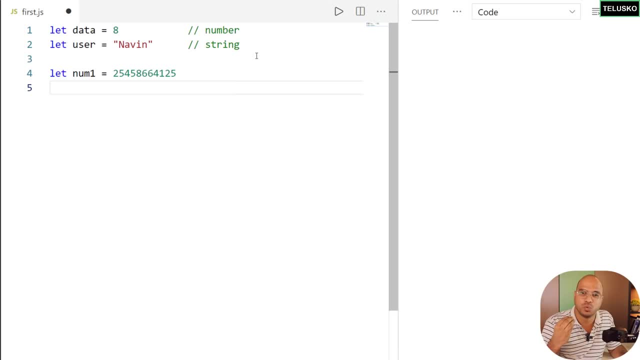 numbers right. We calculate, we perform operations. Maybe you want to multiply, subtract, you want to find the percentage. whatever operation you want to achieve, you can achieve that with the help of a number type. So what are the operation talking about? So I'll simply say num1, n2.. So, whatever variable you have, 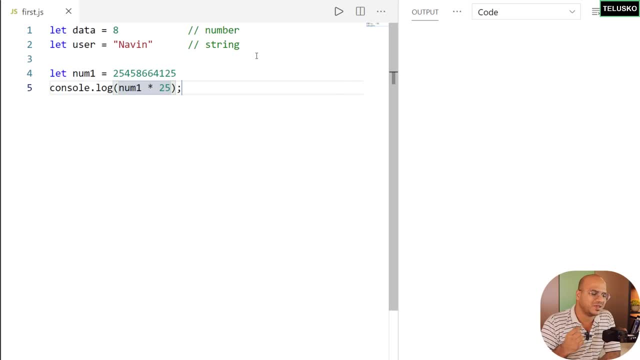 I can perform operation. Let's say I want to multiply that number with 25.. Now the only problem is: how do you verify if this is correct? Okay, let's try this, Let's see what happens. So I will go to my terminal And here I will say: first of all, I will say CLS, so that it 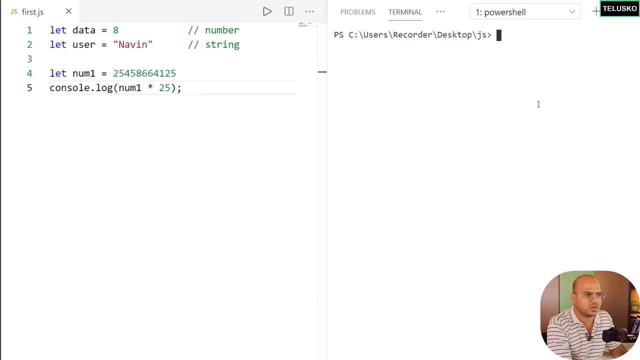 will get empty and i will run this. so i will say node first, dot js, and when you say enter you can see we got the output. the only problem is difficult to verify. but then it says 25 into 25 it's 125 at the end. we can trust that number. so you can use calculator as well. but this, this works. but then 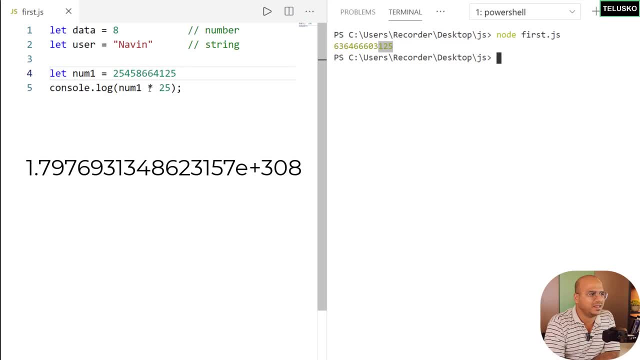 how long this number can be. there should be a range right now on this screen. this is a range with a number. you can have any big number of this range. right and mind you, it's a power of 10, so this is a length you can work with, but the only problem is if you have a bigger number, very big. 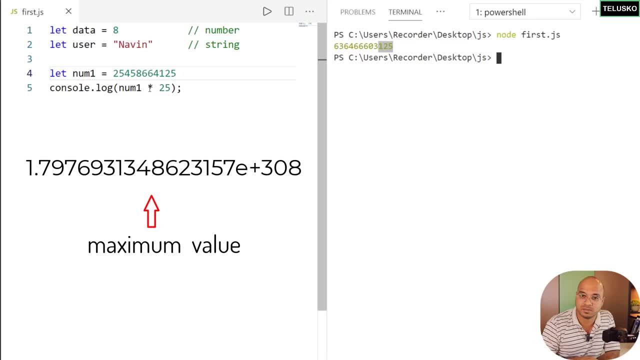 number, it might have some inconsistency with the numbers. so the safe integer range or safe number range is this: if you have your number between these numbers, then you will not be having any issues of data consistency or number consistencies. but then you'll be thinking, hey, what about if you? 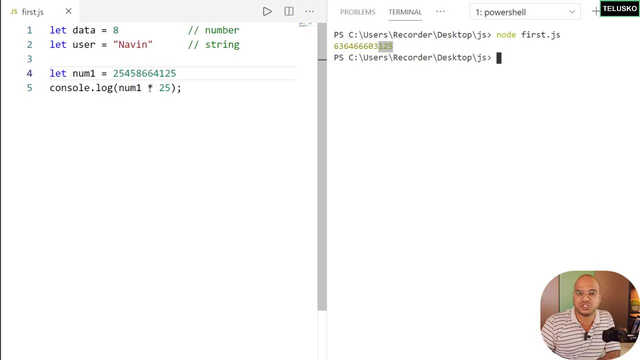 have a number bigger than that. in that case we have a very special subtype of number which is called big int. big int: it was not there in javascript from earlier stage. it came later and that's why in most of the project you still work with normal numbers. but yeah, we'll talk about big int as well. okay, so you got this. 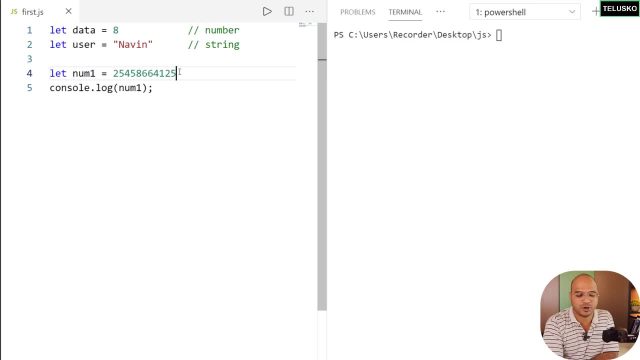 number right and we are able to work with it. but what if you have a decimal point here? so what if i say a big number, dot 8, will this work? now, this type of numbers in number system is called floating point representation. so when you have a decimal number, we say floating point. so let's. 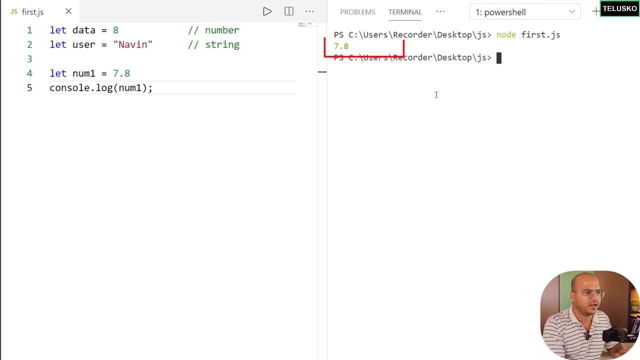 say 7.8, just to make it simple. and if i go back here and if i run this code, you can see we got 7.8. now is it a normal number? yes, so this is a number. so by default, all the numbers are represented in floating point. so even if you use a 7, it's 7. 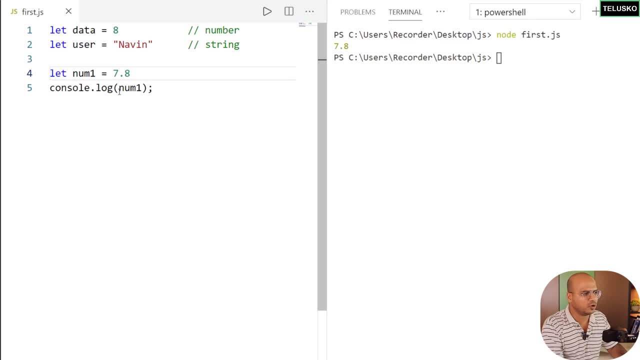 points, although you can imagine. so 7.8 also works. there is one more operator which we're going to talk about. so what if you want to know the type of value? so, example, when i said this is a number, this is a string. what if i want to know the type in the output? so there is a special operator called 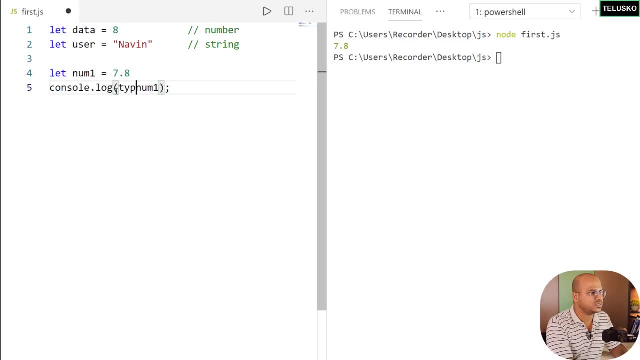 type of. so let's use type of here, so we'll say type of. it's an operator and you just have to pass a number. so mention the operator name and the variable name. so type of the variable name, number one, and let's see what happens. so if you run this code you can see it says number the same thing. you. 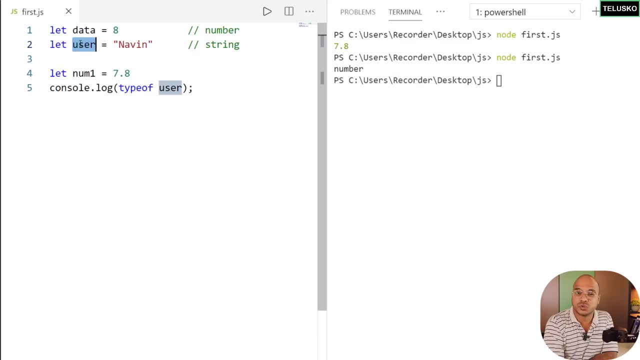 can do with user. now. if you look at user here it's a string right, and now i hope i have saved it. so if you run this code now you can see we got string. same thing can be done with any other type which you have used this in the process. so so it's. 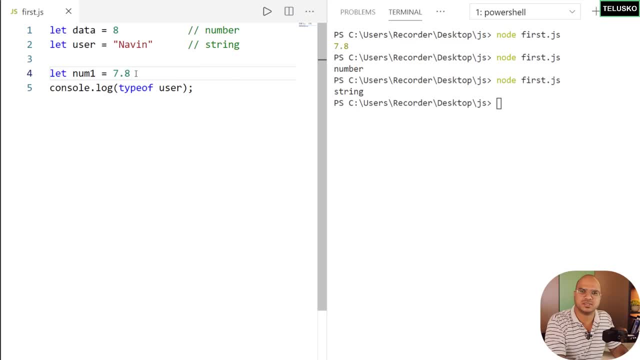 also there really good in this video. how works f, f, f, f, or maybe 0, 0, 0, 0 or 0, a, o, f. so we do that right example here. i want to represent the number with the help of hexadecimal. the way you can represent that is by specifying 0 first. so say: 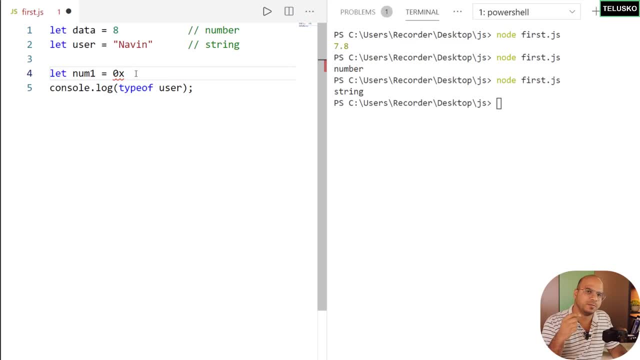 say 0 and say x. now, whatever you mention after this will be a hexadecimal number. example: i want to say f, so f is actually 15, the last number in hexadecimal, and let me just print the number as it is. so i will print num1 and let's see what's the output you are getting. so we got 15. this is 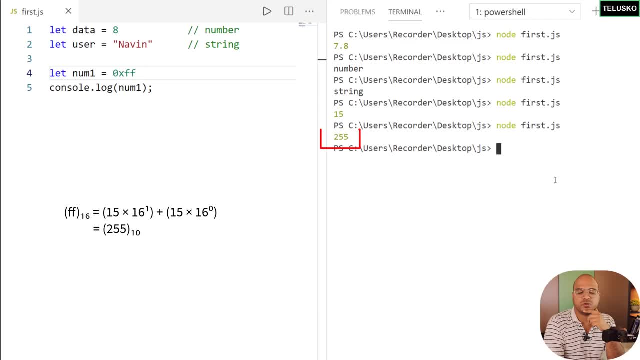 working. what if you say f, f, now this is 255. so you can see the calculation. so this is 255.. in fact, there's one more thing with the number system. you can actually represent floating point with the help of e exponential example. when i say 1.5 e, let's say 12.. now this is actually exponential. 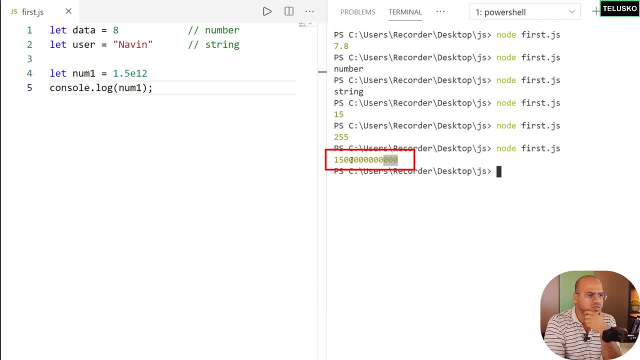 you can also represent this and you can print and you can say: we got the value. so this is the exponential, so it is 1.5 into 10, raised to 12, and this is the output you got simple. we can actually have one more fun here. 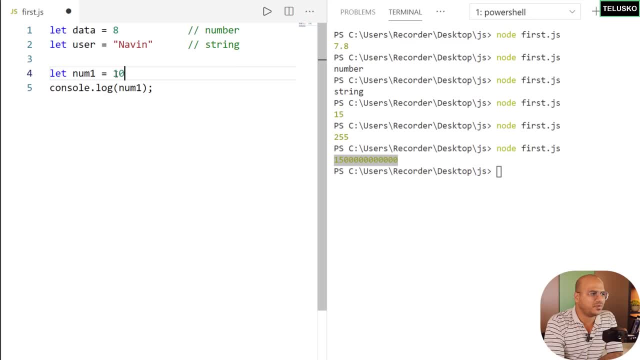 you know i have this problem. i don't know if you have this issue, so whenever i type amount. so let's say, if i want to transfer 1000 rupees, so 1000 is easy because we have only three zeros. what if you want to transfer one lakh rupees? in that case you mentioned five zeros, right, and you verify it: ten. 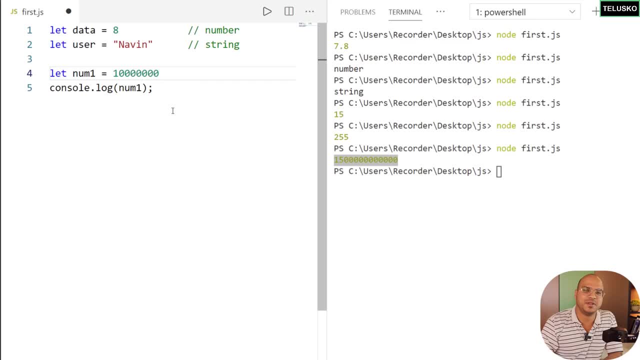 times do i have exactly have five zeros, or? but if you have a very big number, so let's say you have seven zeros or eight zeros, i'm not even sure how many zeros we have on the screen now. so do one comment how many zeros you can see. i don't think only i have that issue and that's why we got a new. 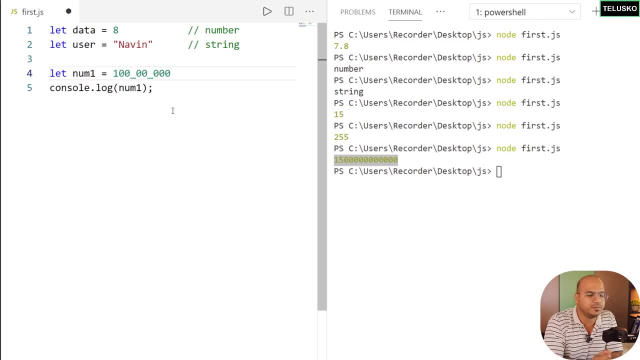 feature, not a new feature- but you can put underscores in between numbers so that you can differentiate it. and is it read right? so now it says: one, two, three, four, okay, seven. there are seven numbers, seven zeros there, only underscore. yes, you can't use comma there. okay, the way you. 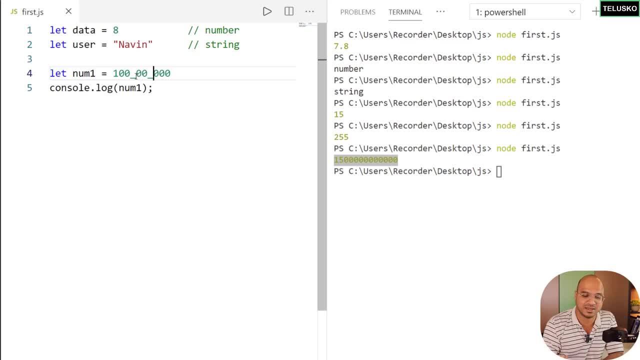 do it. in real world. you can't use comma, because comma has a special meaning in javascript. okay, this is working. the other thing you can also do is you can work with infinity. right, it's a type of number. so you can see, comma is actually a very big topic, so we are focusing more on that. so let's. 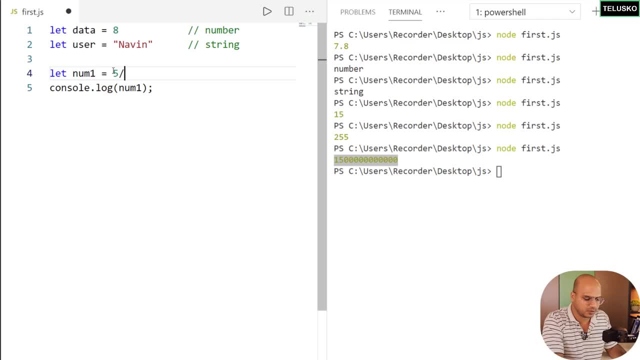 say, five divide by, and we all know, whenever you divide a number by zero, what you get is infinity. but do you really get infinity or do you get some weird answer in javascript? let's see. so if you have this code, we literally got a type which is infinity. so infinity is a type of number in a 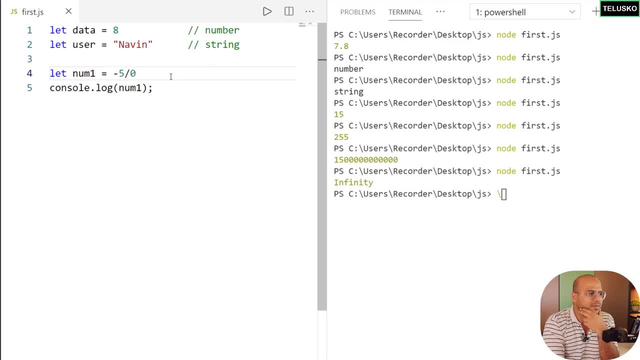 subtype. okay, what do you think if i divide a negative number by zero, what do you think what will happen? so basically, we have a range of positive infinity and negative infinity. so you mean not just this, you actually have a maximum value in the number system, right? so i can say: 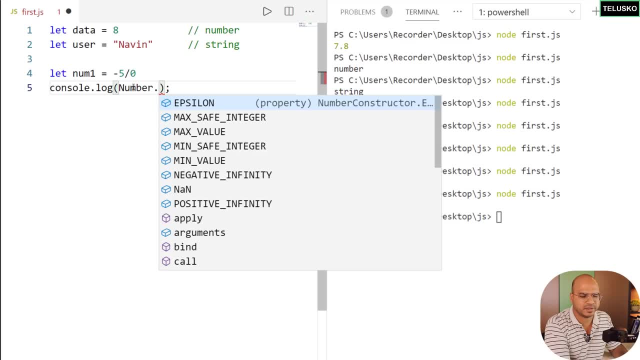 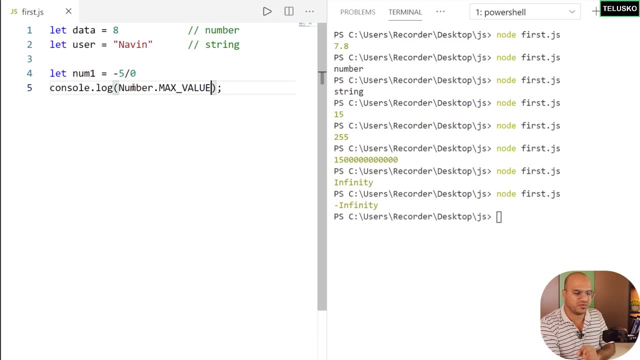 number. so we have a special interface called number. we'll talk about that in detail later what this number means. but imagine: this represents a number. so when you say number dot, max value, so this is a maximum value you have which you can use, and let's print this and let's see what happens. 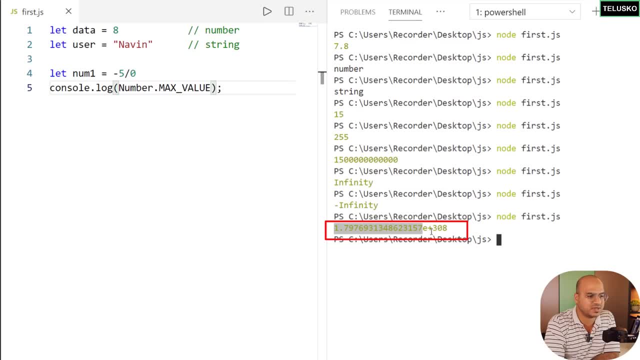 so when you run this code, this is a big number. remember, this is something which we have seen earlier: bigger range. now, if you have a bigger number and if you say plus 10, let's see what happens. plus 10 should work, i guess. let's say, multiply by 10, so the maximum value multiply by. 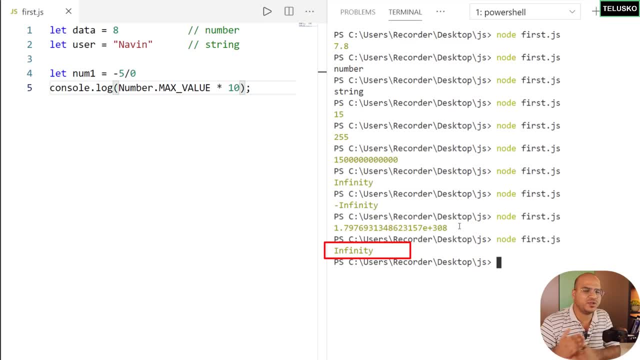 10 and if you run this code you can see we got infinity. so when you go beyond a maximum value, you get infinity. same thing can be done for the negative infinity. if you want to go with, maybe you can try min value and divide by 10. so that should work. okay, enough of fun with a numbers. 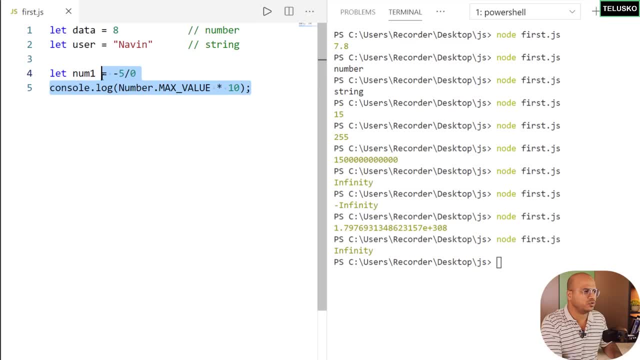 there is one more, one last. what if you have a very big number? you want to represent example here? i have a very big number. i'm not sure if this is a really big number. you want to represent example here? i have a very big number. i'm not sure if this is a really big. 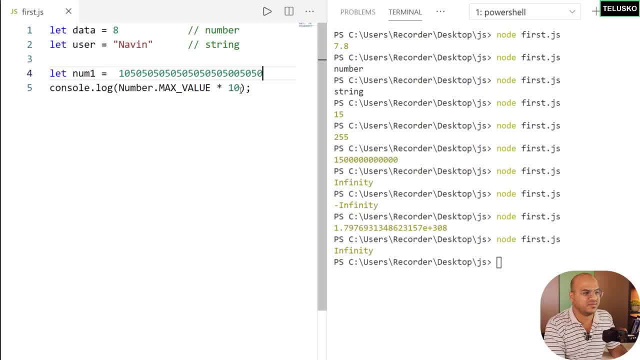 number which will not be supported by javascript. i don't even know how many five zeros i'm typing there, i just want to print. no one, and sometimes you learn by doing stuff right. so let's do it, let's try. and oh, it's working. so it does support this big number anyway, so you can try. begin the. 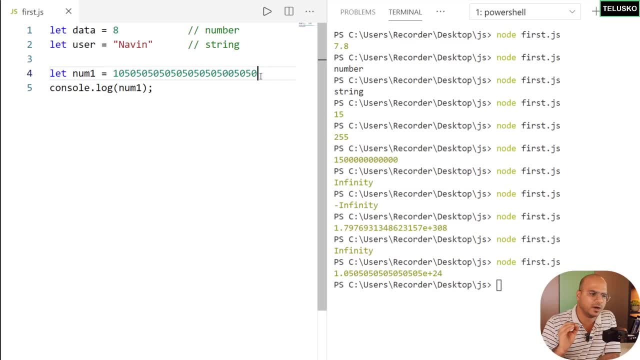 bigger numbers here. what's important is if you have a bigger integer and if you don't want to lose any precision example: i guess i'm losing position here. if i say one at the end, i run. can you see that we are actually losing data? it says a number and then 10 raise to 24.. which 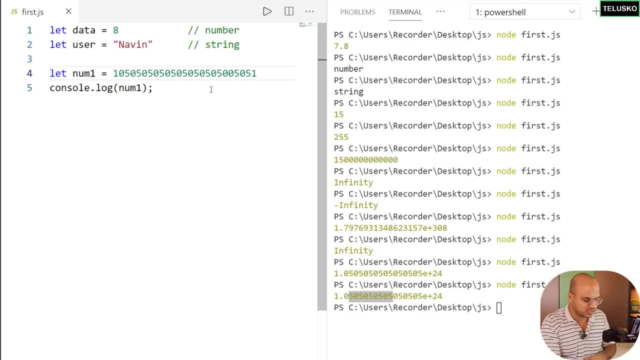 we don't want that. what we want is we want one as well, so you can also represent this number with the help of big n. so just give a n at the end and this will represent it as it is. so this is big n, a special type where you can have a bigger number. so just say n at the end. the only caveat here is: 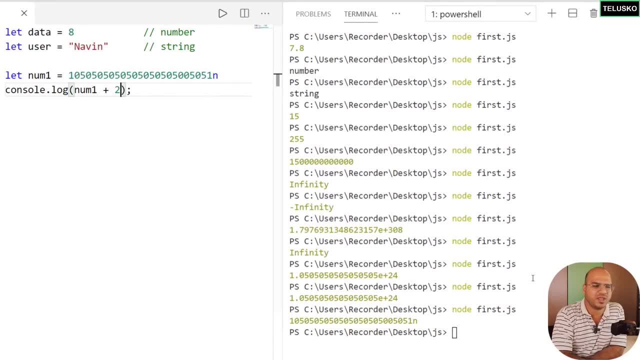 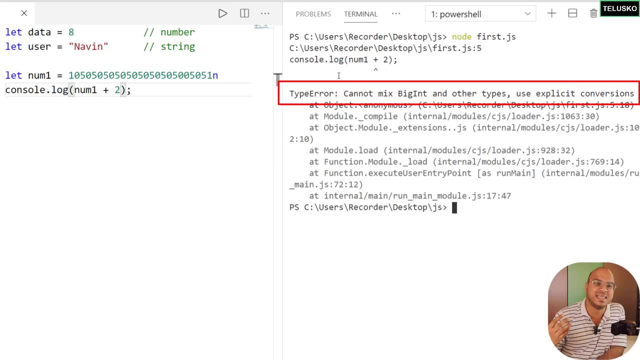 if you add this number by any other number, let's say two, what do you think what will happen? this will give you an error. why is? because it says okay, as i mentioned before, it's very important to understand the errors right. so it says: cannot mix big ain't. 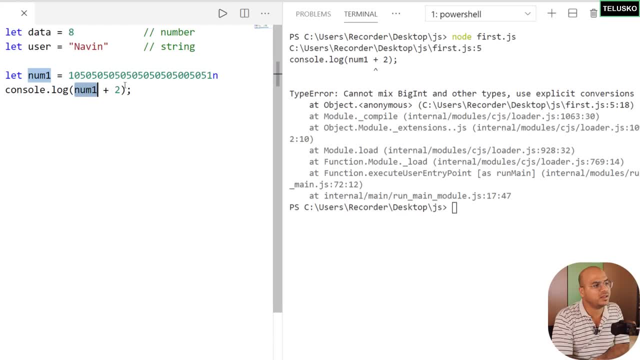 and other types. oh, this is big integer, now one, and this is a normal number. so in this case, if you want to perform the operation, you can simply say 2n. again, we'll talk about how do you convert this. maybe you can convert this to into a big integer, or maybe you can convert this. 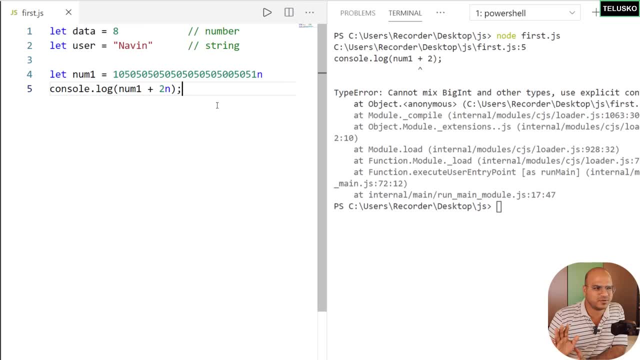 number into normal number. so this option of type conversion- we will talk about that in a separate video. okay, as of now, this is working. so you can see we got 53 at the end. so that's how you can work with big int. okay, this is working properly. now i know there are some curious minds. they've 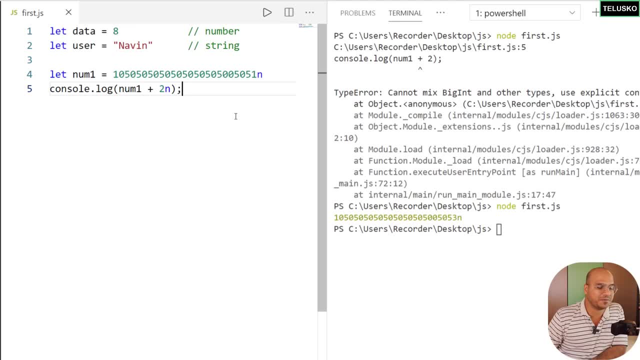 got a lot of questions, so i want to know what is happening behind the scene, how everything is working behind the scene. we'll talk about that in a separate video. as i mentioned before, we are here to learn javascript from start to end, so somewhere in between, once you know the basics, we'll go with. 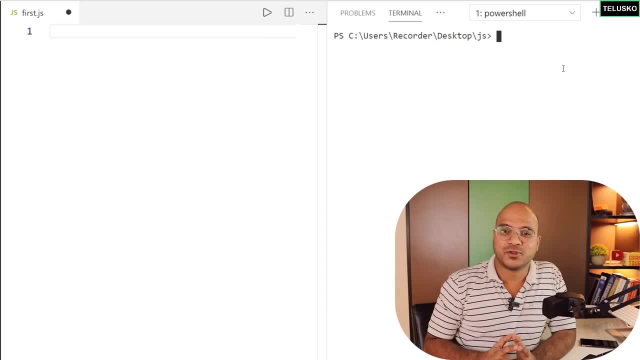 advanced part, where we'll know how things are happening behind the scene. very important, right? so, basically, we have talked about the data type. so we have two categories: we have primitive and we have object, out of which, in primitive, we have talked only about numbers. in the next video we'll